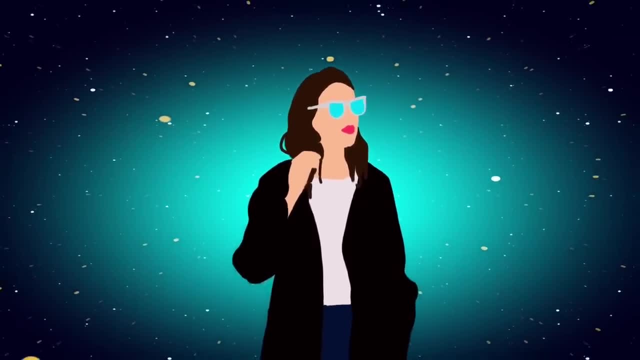 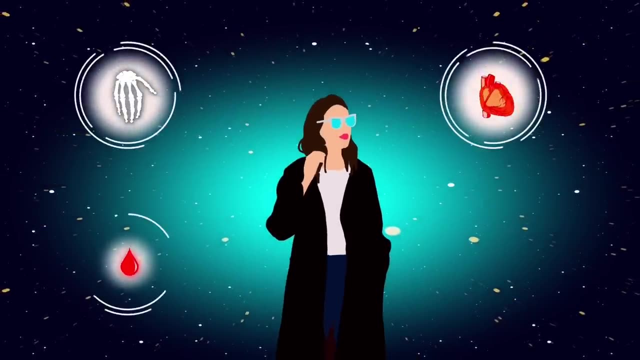 We humans are the most intelligent creatures known to have ever appeared in the universe. What are humans made of? The human body is composed of organs, bones, blood, nerves and more. Take one of the organs, the heart. And if we zoom into it deeply, 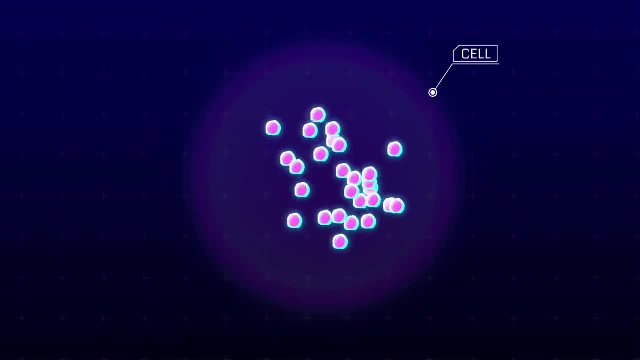 we can see billions of cells, But the cell isn't its final stage. Again, if we zoom further into a singular cell, we'll end up with molecules. In just this one cell there are millions of unique, complex molecules. Take one of these molecules, zoom in even more and finally we 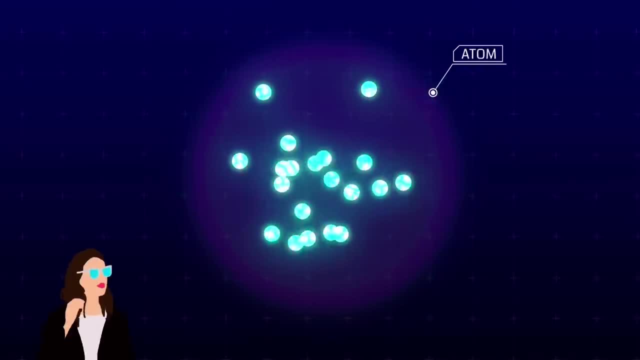 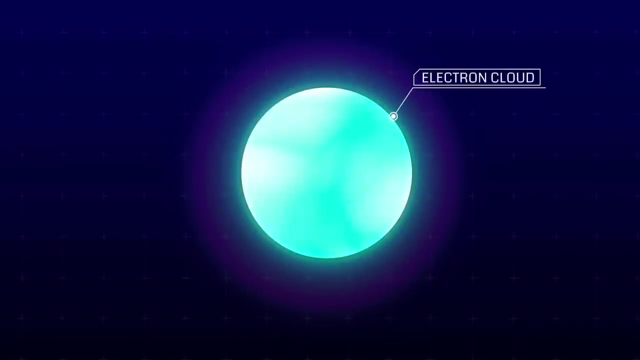 can see atoms. To put it simply, the human body consists of around 40 trillion cells, and a single cell contains approximately 100 trillion atoms. But atoms are not the end of the story. If we could magnify more, we would see clouds of electrons at the outer edge of the atom. 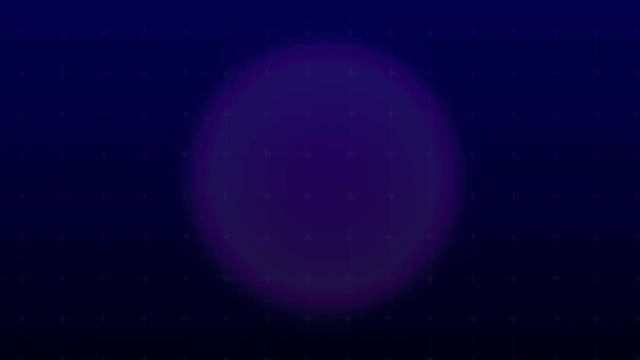 and if we magnify again, we will end up with empty spaces. But let's not just stop there. If we keep zooming in, we will see a cluster of different atoms, and then we'll only see one. If we keep zooming in, we'll see a cluster of different atoms, and then we'll only see one. If we 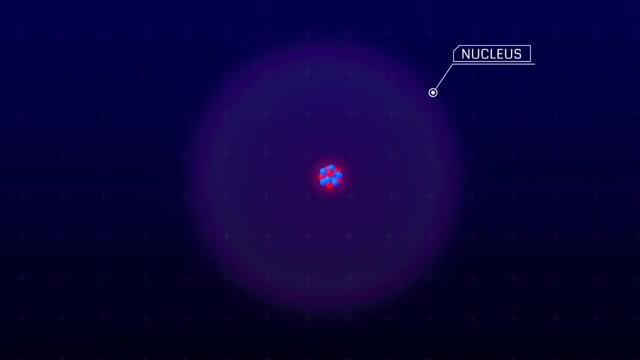 further at the center of the atom, we would see the nucleus. Yes, the orbiting electrons and the nucleus are collectively called an atom. But again, the nucleus is not the end of the story. If we zoom further into the nucleus, we will see protons and neutrons. 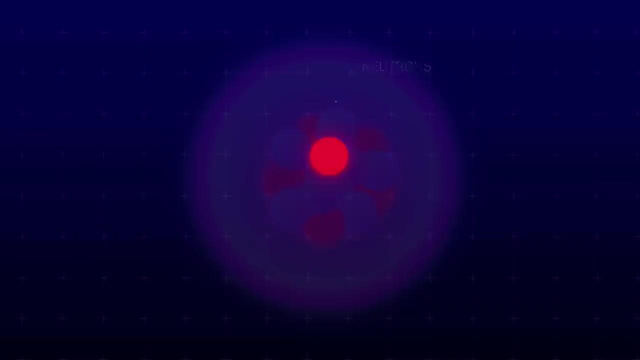 sticking together. These are subatomic particles. Let's take one of the protons and again zoom into it. Inside the proton we can see tiny dancing particles, These quarks. these tiny particles, are called elementary particles or fundamental particles. Quarks are elementary. 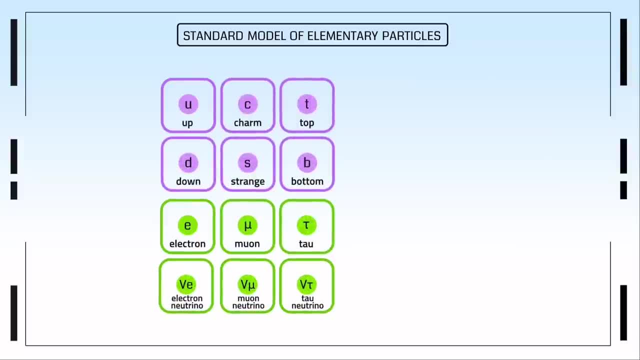 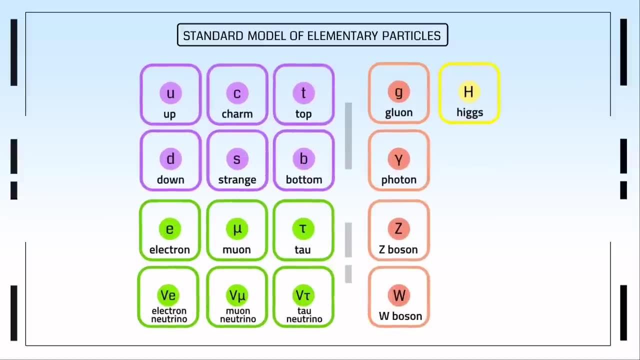 particles, But there are a further total of 12 matter particles and 4 force carriers in the standard model of particle physics. So what classifies something as an elementary particle? If we look at the proton, it consists of three quarks. However, it is more precise. 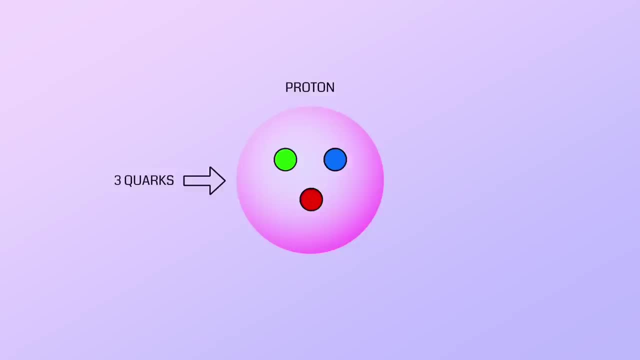 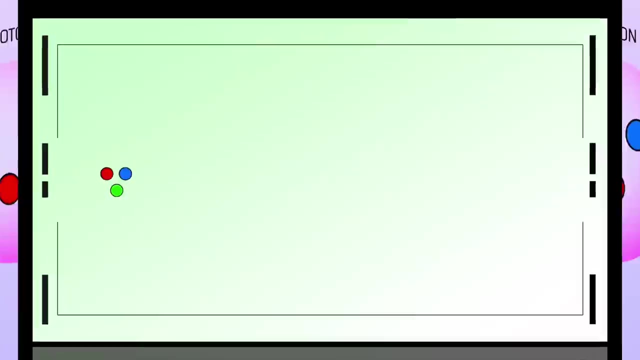 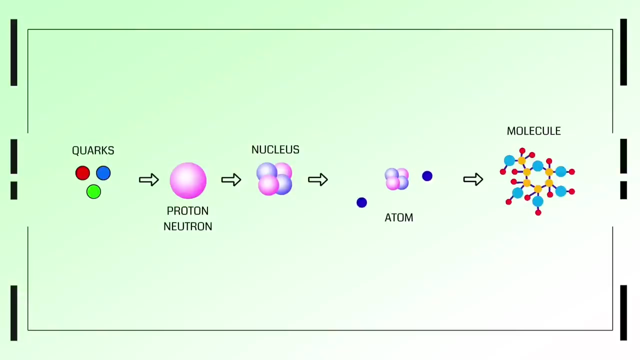 to say quarks collectively form a proton, rather than a proton contains three quarks. So protons are not elementary particles, They are subatomic particles. Elementary particles don't have any substructures and cannot be broken down into smaller components, which means they aren't made up of anything. 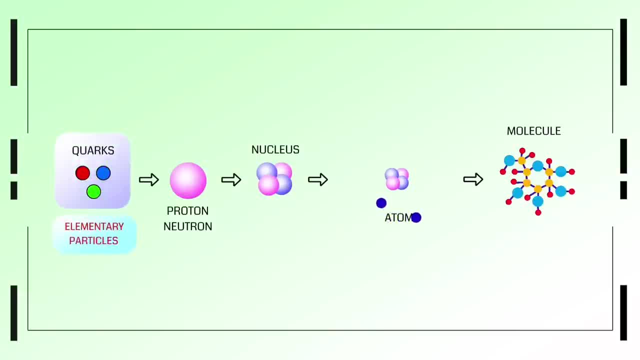 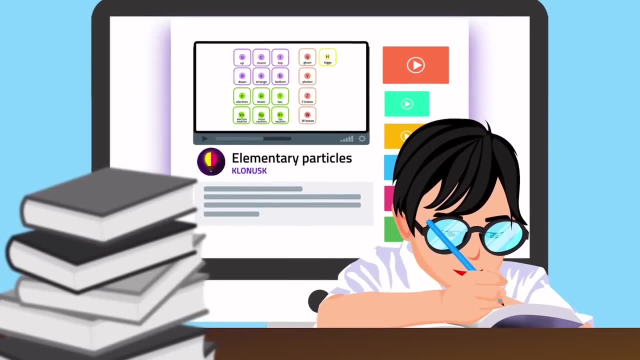 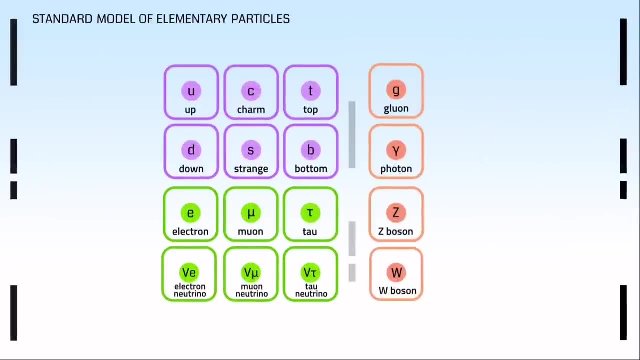 These are the final and smallest known building blocks of our universe. The study of elementary particles is called particle physics. Studying and understanding these particle forms the foundation of both classical and quantum physics. So let's return to the standard model. There are 12 matter particles and 4 force carriers. 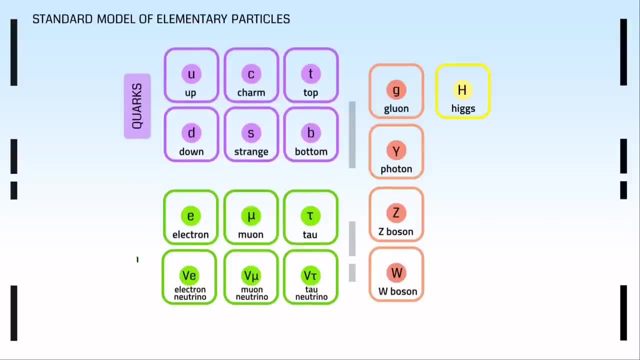 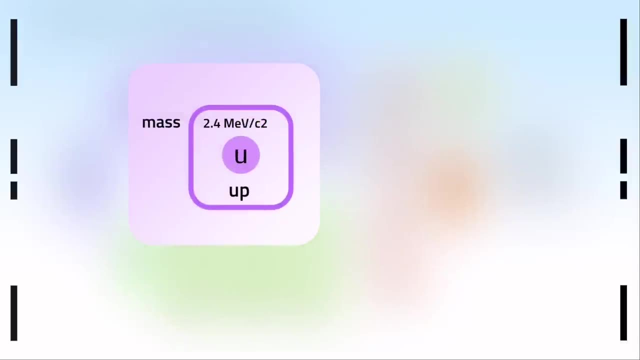 They are classified into three families: Quarks, leptons and bosons. Quarks and leptons are together called fermions. All elementary particles have three basic properties: Mass, spin and charge. If we look at the first particle, it has a mass of 2.4 mega electron. 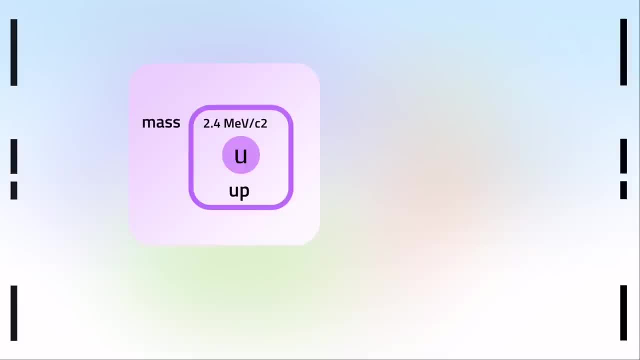 volts divided by c squared. Mass of an elementary particle is mentioned as energy. It comes from Einstein's mass-energy equivalence equation E is equal to mc squared. For example, if we convert 1 gram of mass into pure energy, it becomes 5.6 into 10 to. 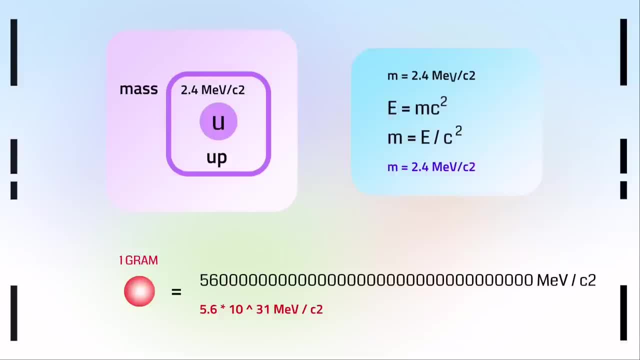 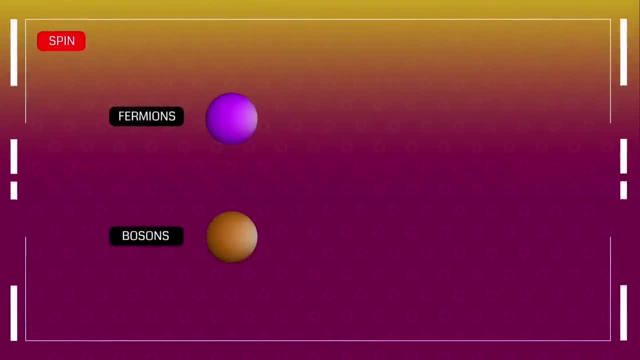 the power of 31 mega electron volts. So from here we can compare the mass of this particle with 1 gram's energy. In the realm of particle physics, fermions are generally characterized by half-integer spins, while bosons typically possess integer spins, such as zero, one or 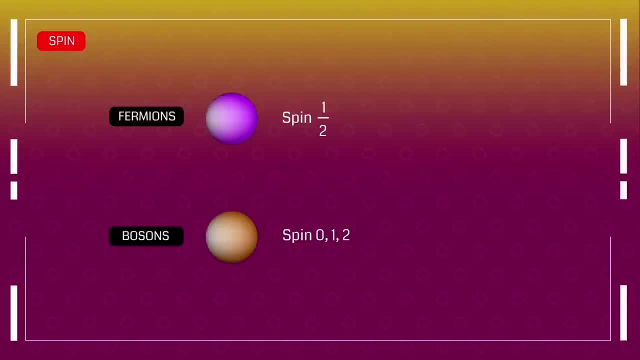 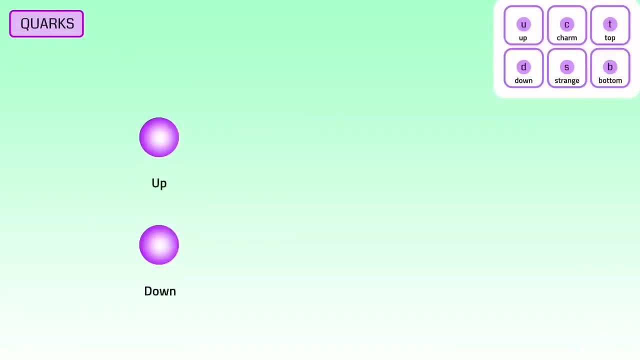 two. However, be careful. Although we use the word spin, it's not the same as the spinning of a ball. First, we start with quarks. There are up quarks and down quarks, and each of them come in three generations. so in total we have discovered six flavors of quarks. The up quark has a. 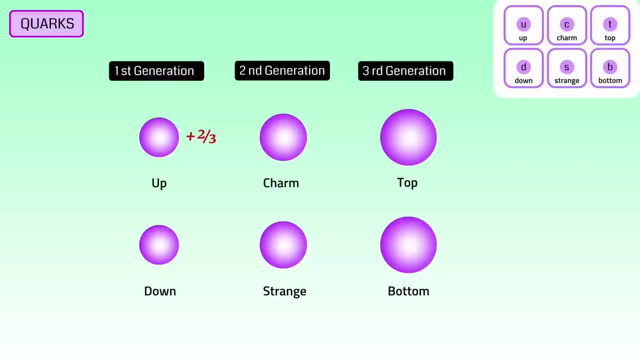 charge of plus two-third, while the down quark carries a charge of minus one-third. This same charge is continuous in their subsequent generations. There is no major difference between the generations, though each generation tends to be heavier than the previous generation, because when the first quark carries a charge of minus one-third, the second quark carries 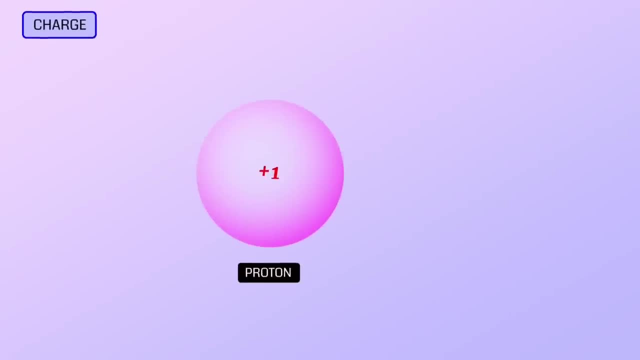 one. We've already heard that a proton has a positive charge. That charge is simply composed from the charges of the quarks. A proton is composed of two up quarks and one down quark, So the combination of charges comes as plus two-third, plus two-third, minus one-third. 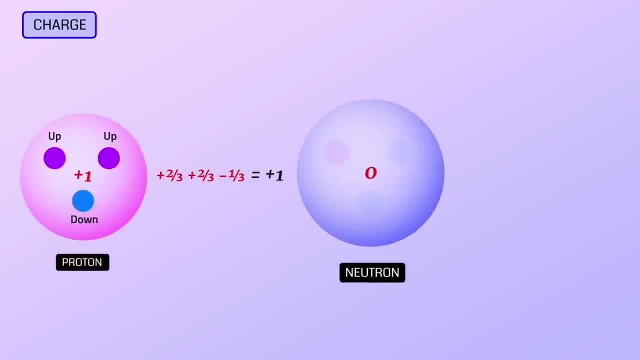 which is a total of plus one. Similarly, a neutron is composed of one up quark and two down quarks, and the combination of charges minus one-third minus one-third plus two-third totals zero. So the neutron comes with neutral charge. The combination of three quarks is called a baryon. 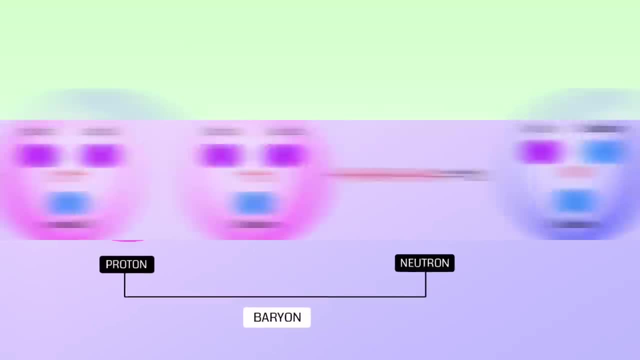 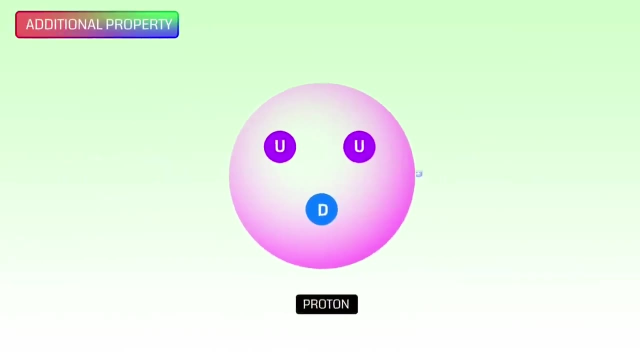 Therefore protons and neutrons are baryon particles. Now we can see that the same flavor of quarks exist in a single baryon particle. For example, a proton has two up quarks. Now how do we distinguish them? That's where an additional property comes. 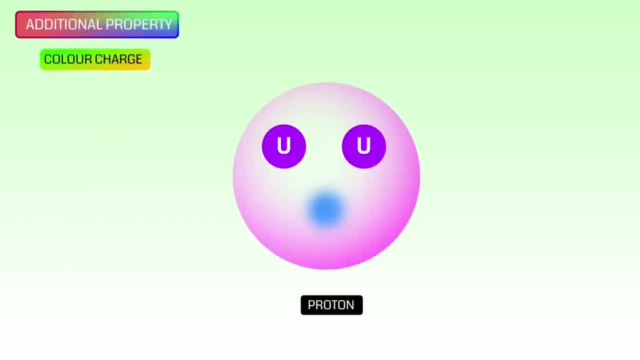 into play, which is the color charge property, And how do these three quarks bind together? It's also related to the color charge property of quarks. Each flavor comes in three colors: red, blue and green. However, don't let these colors mislead you. Quarks are much too small. 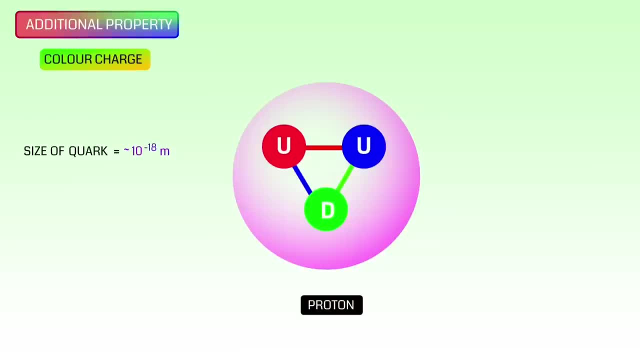 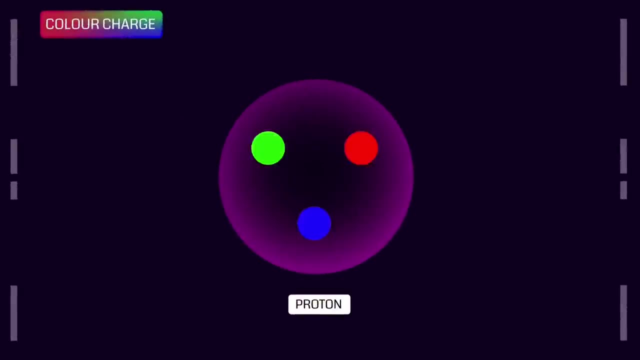 to be visible and thus could never have a visible property-like color. The names were chosen because of a convenient analogy. In a proton there are three quarks and they constantly exchange colors among themselves. But how do they exchange colors and interact? That's where the messenger particle or force carrier, gluon, comes into play. Quarks- 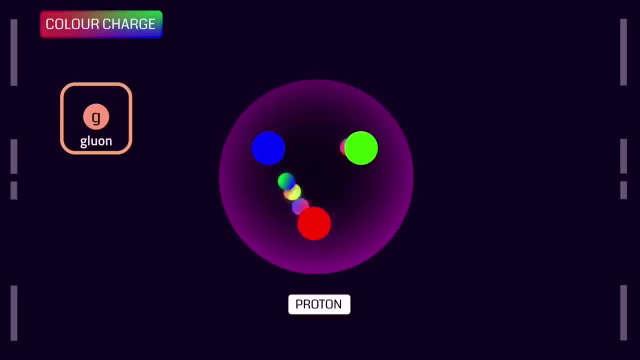 are able to change their color during their interactions. The gluon acts as a messenger particle, carries a color charge from one quark to another and facilitates interactions between quarks. So gluons hold quarks together by exchanging color charges. Since gluons are 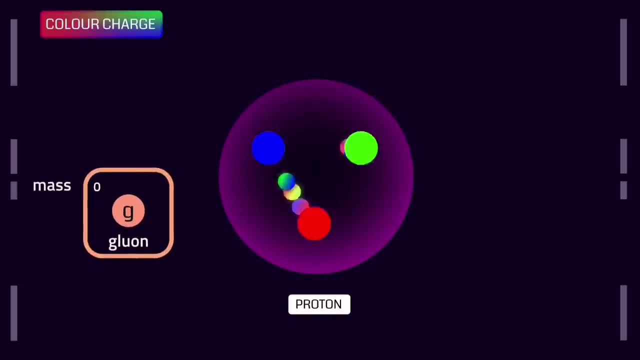 massless. they exchange colors between quarks. However, the same color cannot exist simultaneously in two quarks, For example, in a proton. if one quark has a red color, the remaining two quarks will have green and blue If one quark has a green. 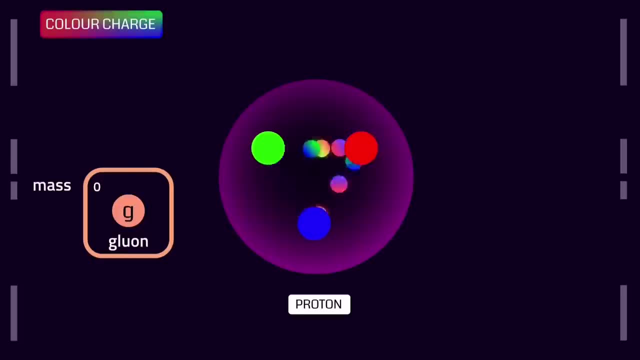 color. the other two quarks will have red and blue. Thus three quarks in a baryon particle always have different colors by exchanging gluons. If we combine the red, blue and green colors, we end up with no color. Therefore the proton is a colorless particle. All baryon particles are. 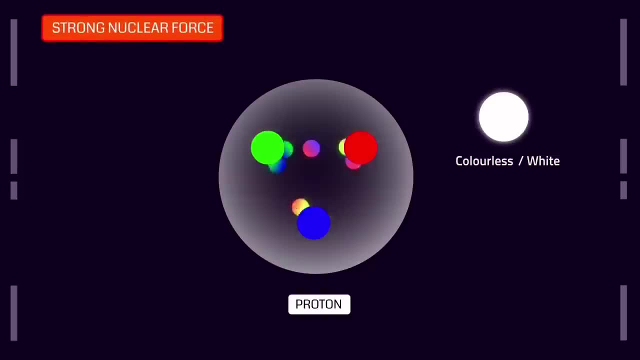 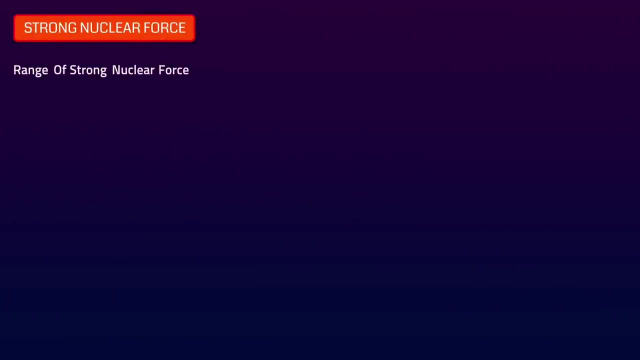 colorless. We've already heard about the strong nuclear force. That force is simply the color charge. that involves the exchange of gluons between quarks, binding quarks together and creating the strongest force in the universe. Even though it's the strongest force, its range. 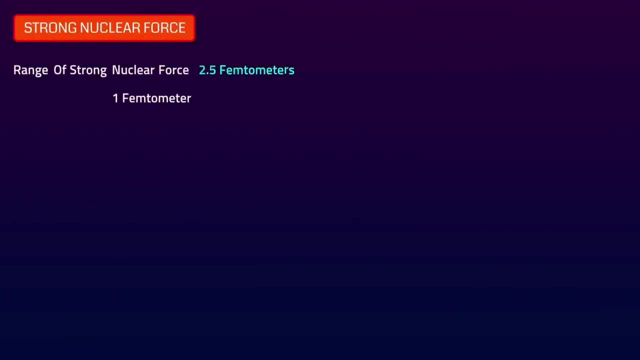 is only a few femtometers. One femtometer equals 10 to the power of minus 15 meters. We've already seen that protons have a positive charge, But how do protons stick together in the nucleus While the same electric charges repel each other and opposite charges attract? 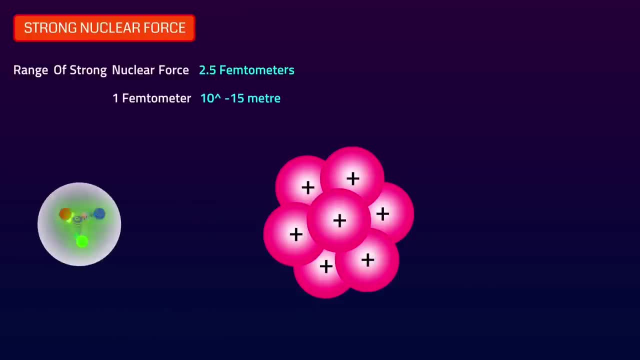 each other. This is also caused by the strong nuclear force. The strong nuclear force can exist within the range of a few femtometers, While the size of a proton is less than one femtometer. the strong force also leaks outside the proton. This strong force overcomes the 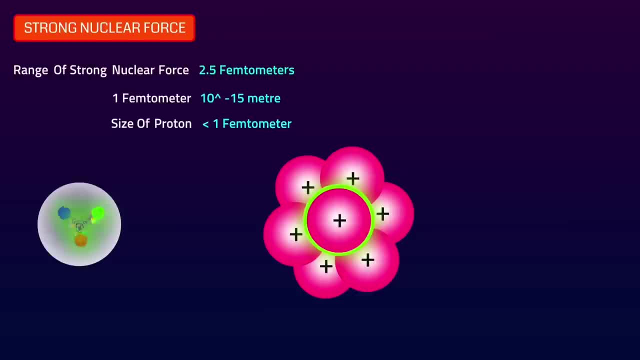 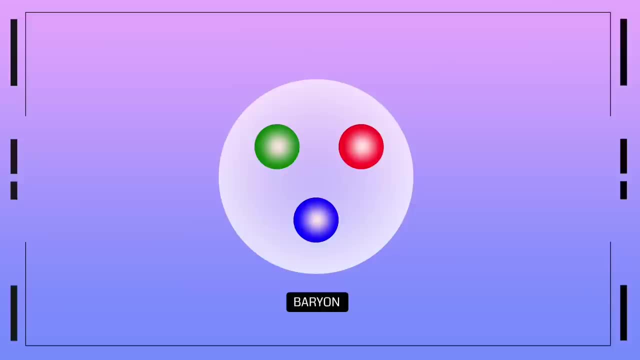 electromagnetic force, so two protons stick together instead of repelling each other. If we try to kick out a quark from a baryon, it requires a lot of energy. Gluons are constantly exchanged between quarks and create a tube-like structure. This tube is very strong When providing energy. 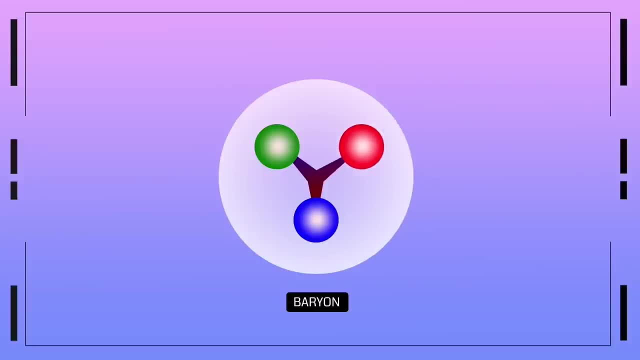 to try to eliminate one quark from a baryon. it acts like a spring or rubber band. The more energy given to pull the quark, the stronger it becomes. But anyhow, if we provide enough energy to remove a quark, instead of kicking it out from the baryon, it creates a new quark. 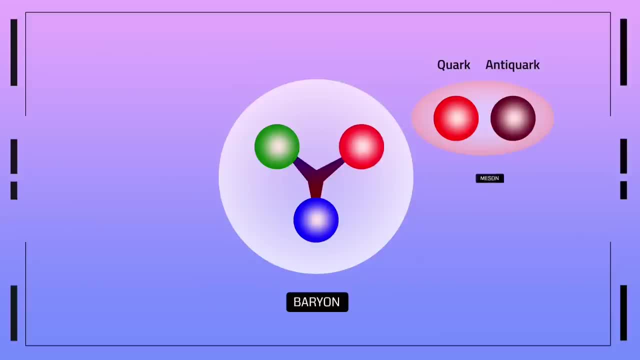 an anti-quark pair. This pair is called a meson. This is how these new particles form and where E is equal to MC, squared comes into play. The energy used to expel the quark from the baryon is converted into mass. 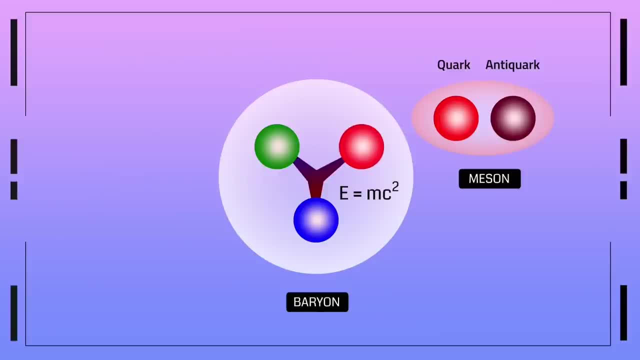 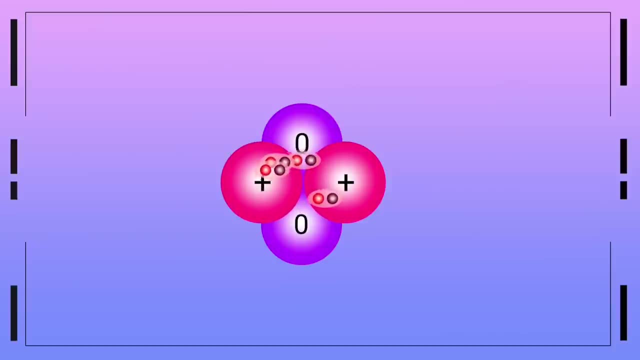 so the extra energy creates a meson. However, mesons decay quickly. The exchange of mesons between two baryons is also responsible for same-charged protons and neutrons stick together in the nucleus. However, we have never found a meson. 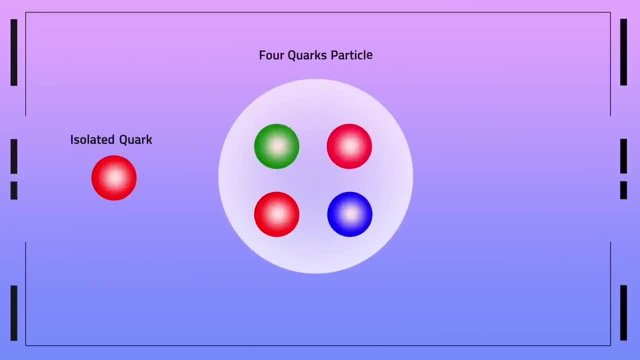 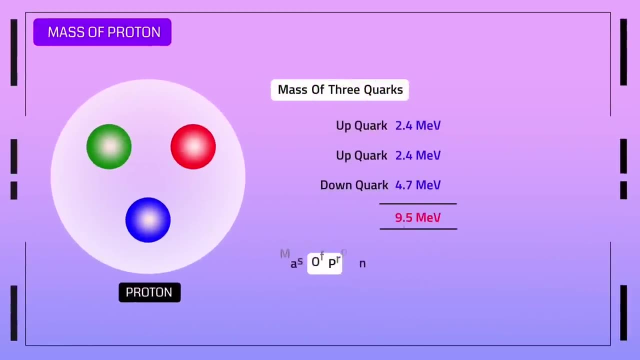 We have never found an isolated quark or a particle with four quarks. And another thing: if we calculate the mass of all three quarks which exist in a proton, they appear to constitute only 1% of the proton's whole mass. 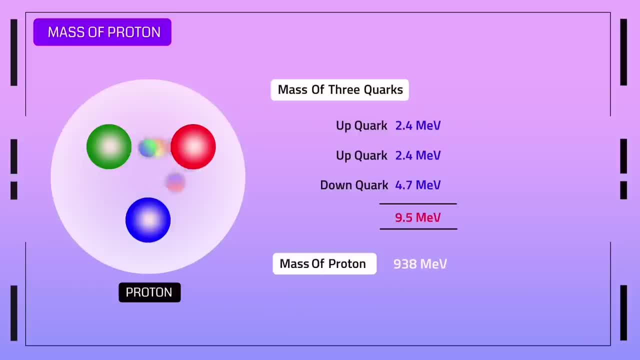 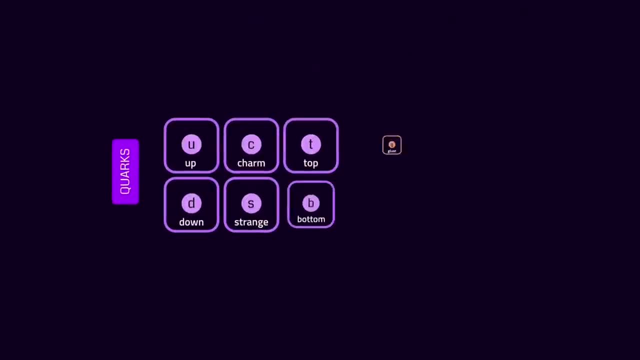 Well, gluons are massless and interact at nearly the speed of light. The energy between quarks converts into mass when we measure it. So far we've looked at quarks, gluons and the strong force which are responsible for creating the nucleus of the atom. 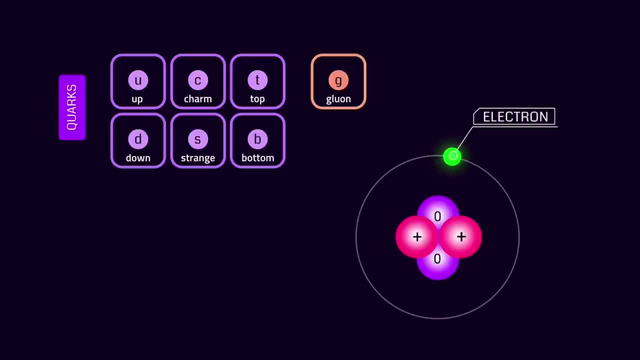 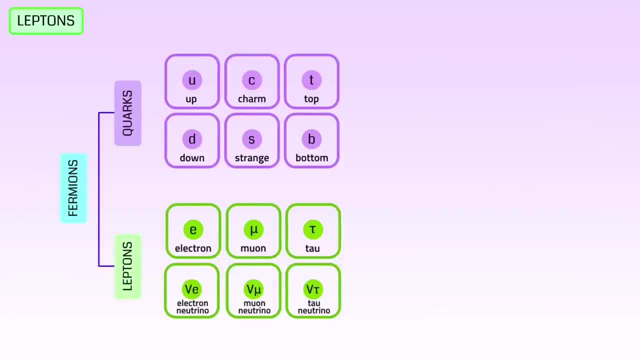 However, an atom contains both a nucleus and electrons. So what is an electron In the standard model of particle physics? in the group of fermions there is another family called leptons. This family includes the electron among a total of six particles. 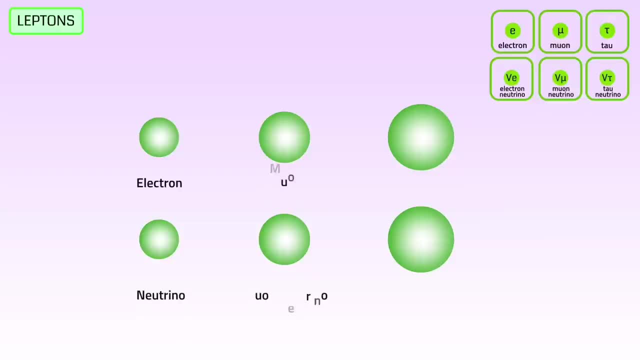 the electron, the neutrino and their next-generation particles. Electrons have a charge of negative one, while neutrinos have no charge. So we can divide leptons into two categories: The charged leptons, which have a negative charge, electrons, muons and taus. 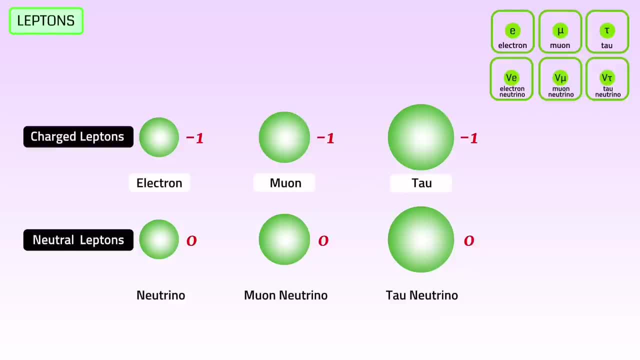 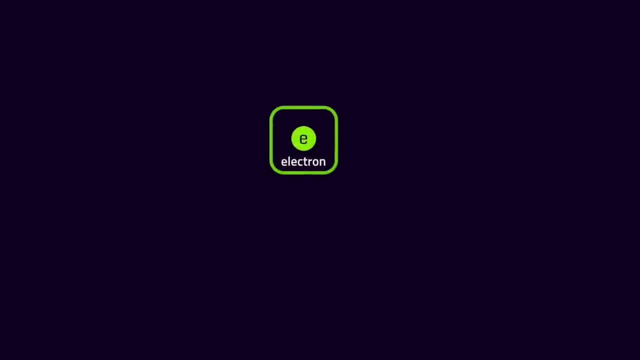 and the neutral leptons which carry no charge: Electron, neutrinos, muon neutrinos and tau neutrinos. The electron is the only member of a family of leptons which is involved in the formation of atoms. Quarks exist only as composite particles. 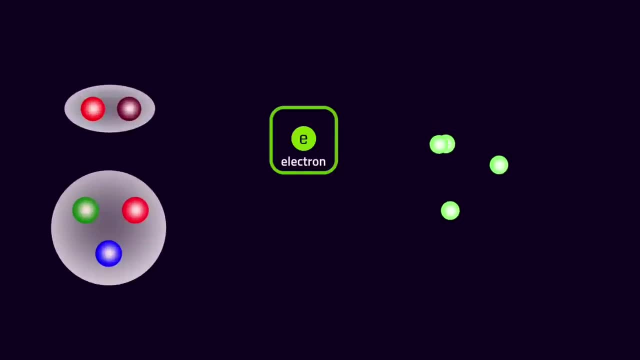 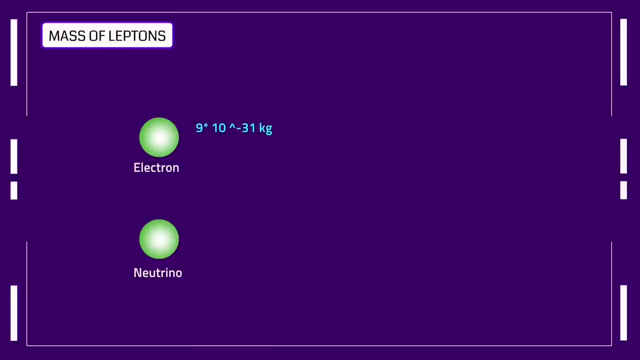 with other quarks, while leptons are individual particles. The size and mass of an electron are very small, approximately 9 x 10 to the power of minus 31 kilograms or 0.5 mega electron volts. However, neutrinos are extremely small. 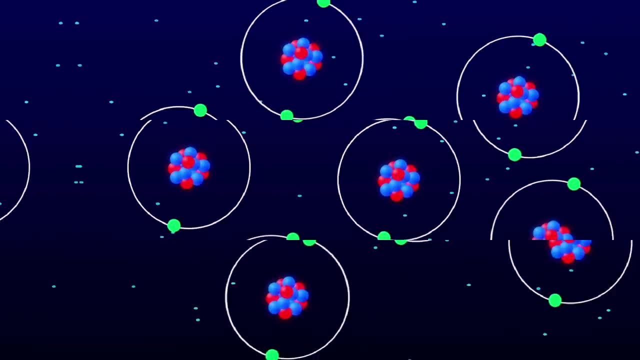 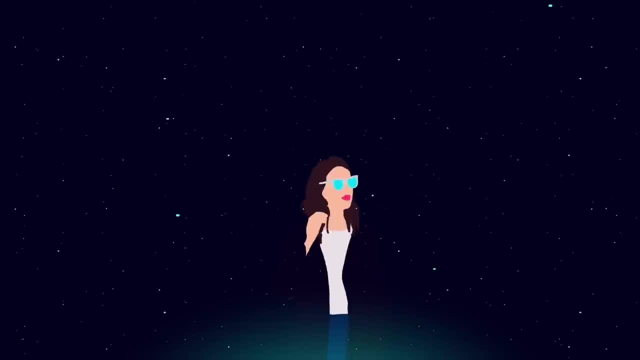 being millions of times smaller than electrons. That's why neutrinos rarely interact with matter. Even though trillions of neutrinos pass through our bodies every second, they are undetectable by modern methods due to their size. Therefore, the neutrino is one of the least known first-generation particles. 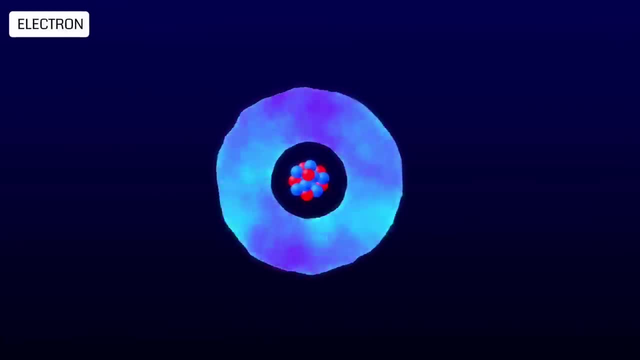 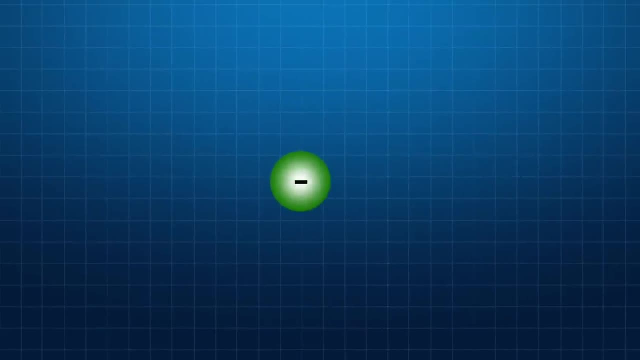 Let's return to the topic of electrons. Electrons orbit the nucleus like clouds due to their wave behavior, but at different energy levels. Electrons carry a negative charge and all charged particles have an electric field. As we already know, protons have a positive charge. 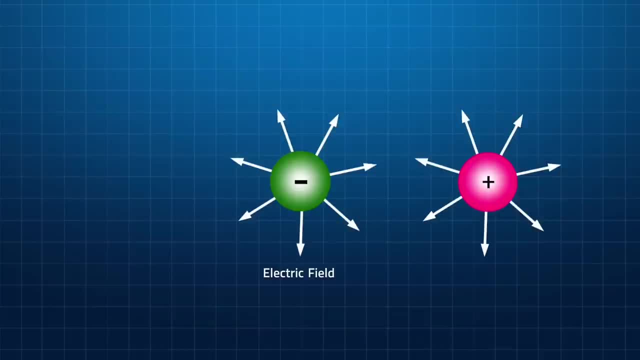 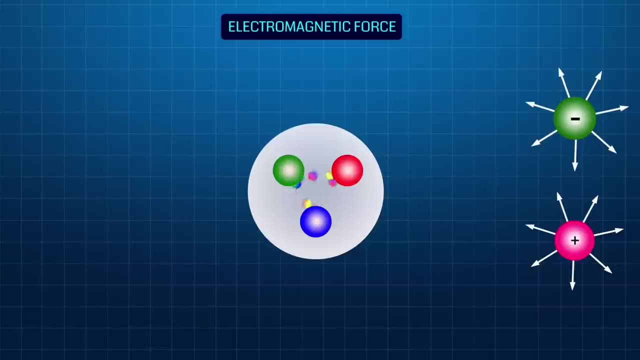 so protons are also charged particles. Then what is the electro-mechanism, Electro-magnetic force? Quarks constantly engage gluons, which are responsible for quarks sticking together, generating a strong force. Similarly, when two charged particles come close to each other, 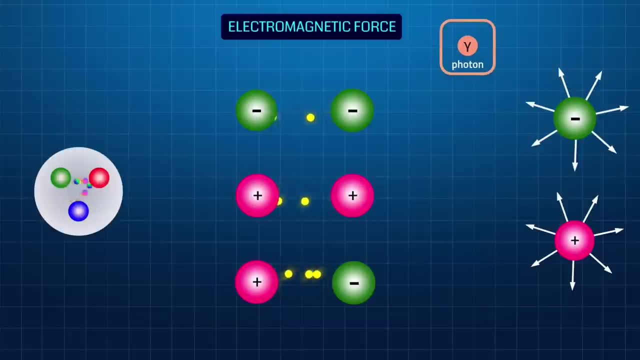 they exchange virtual photons and create electromagnetic force. These are called virtual photons because their energy cannot be detectable. The exchange of virtual photons between charged particles is the reason why particles of the same charge repel each other and particles with opposite charges attract each other. 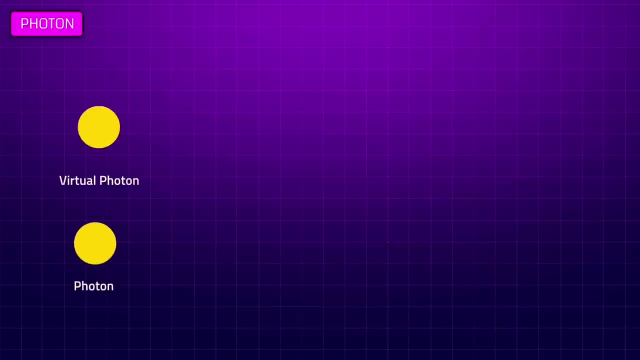 Unlike virtual protons, there are real photons that also carry electromagnetic fields which can be detectable. This is light. We've already seen electrons orbiting nuclei at different energy levels. When an electron jumps to a lower energy level, it emits a tiny packet of electromagnetic radiation, a photon. 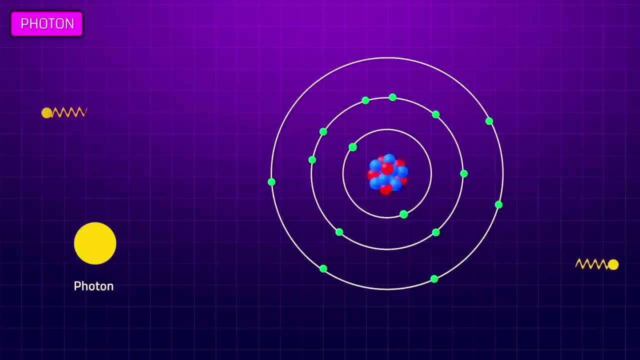 It has no mass and travels at the speed of light. But why do electrons jump between energy levels? Electrons orbit at their own energy levels, but when electrons gain energy it jumps to a higher energy level. However, it is always trying to remain in its original orbit state. 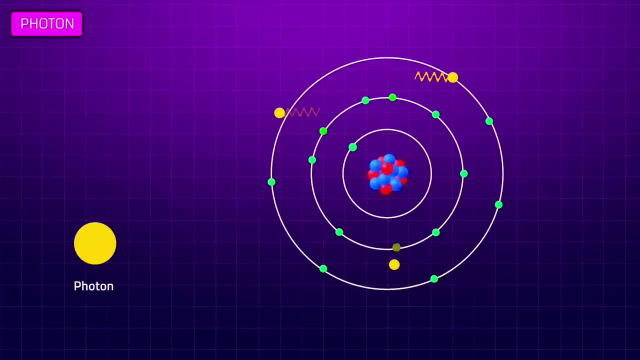 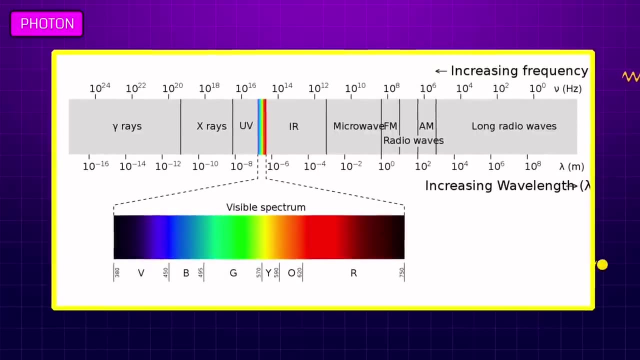 so it quickly jumps back to the normal state. As a result, it releases its excess energy. a photon Jumping between the distances or energy levels determines the wavelength of light. So far we have seen quarks, leptons and their force carriers. 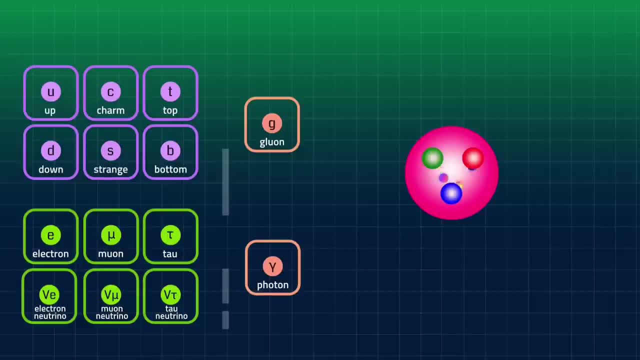 The strong force is responsible for binding quarks together and also for binding the nucleus. Photons act as a force carrier between charged particles, creating the electromagnetic force. The resulting nucleus and electrons attract each other, eventually forming a complete atom. The electromagnetic force is also stronger, but it can never overcome the strong nuclear force. 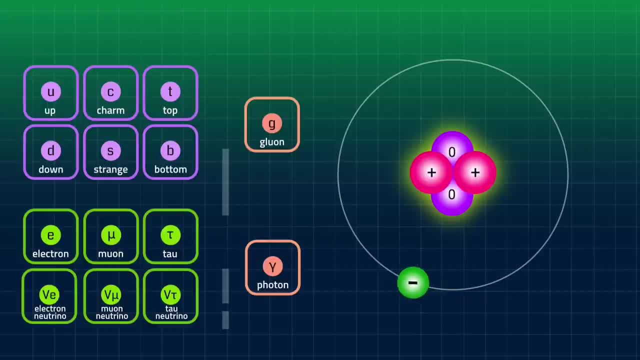 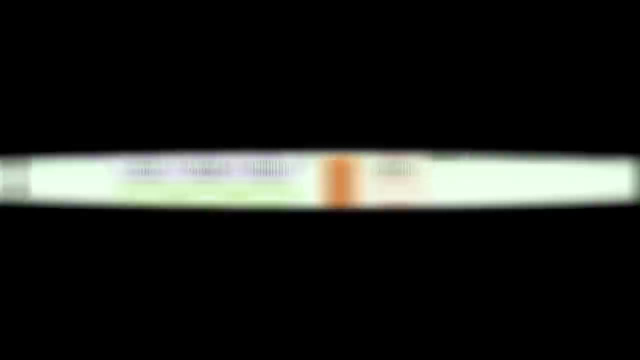 The strong force needs to be strong to overcome the electromagnetic repulsion between the positively charged photons in the nucleus. If it were weaker than the electromagnetic force, no atoms with more than one proton in the nucleus would be able to form. Now we only have two force carriers left in the standard model. 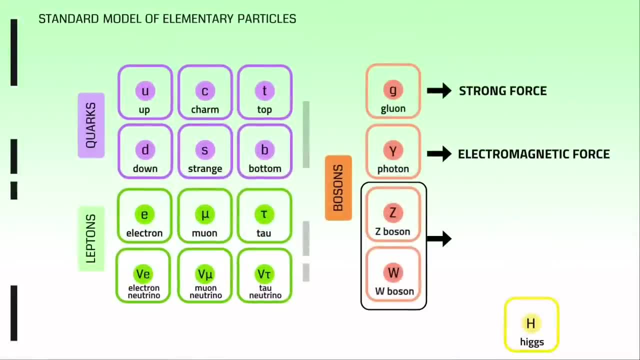 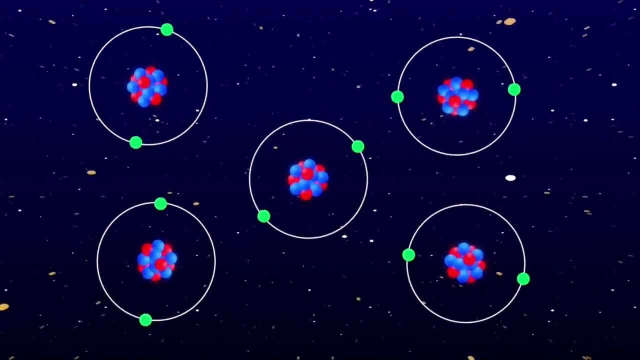 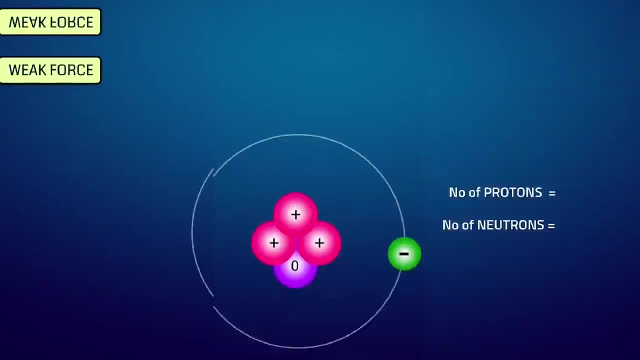 So what is the use of these? It's not very familiar to us, but it's as important as the other forces, The weak force In nature. everything seeks a stable position, So the atom also. What is an unstable atom In an atom, when the number of protons exceeds the number of neutrons? 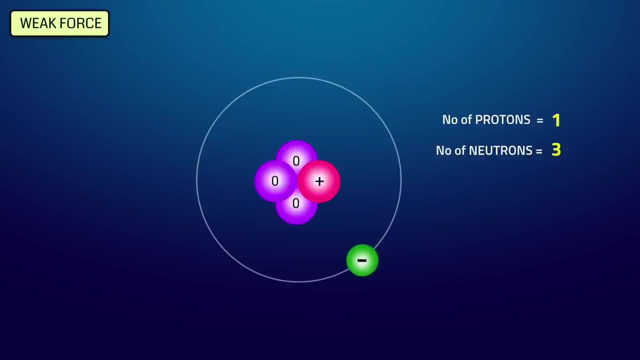 or the number of neutrons exceeds the number of protons, the atom becomes unstable. This unstable atom will constantly try to achieve a stable state. So the extra neutron converts into a proton to maintain the stability of the atom. But how can the neutron convert? 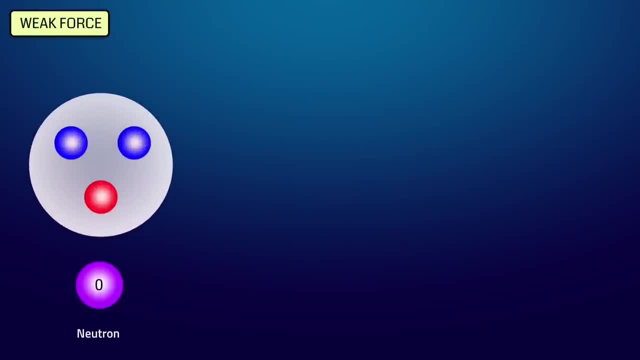 We've already seen that the neutron is a combination of quarks- two down quarks and one up quark- and the proton is a combination of two up quarks And one down quark. So when a neutron converts into a proton, a down quark changes into an up quark. 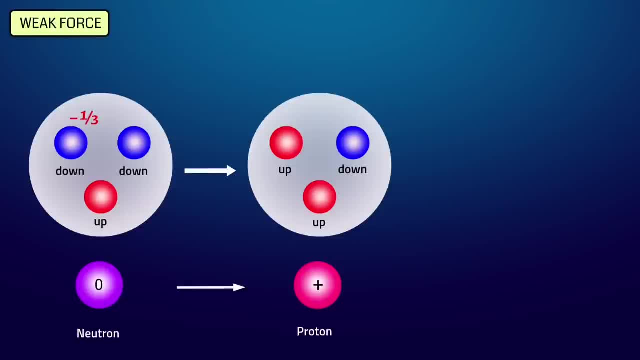 If we look deeply, the down quark has a charge of one done quark And the up quark has a charge of two Telliro quark plus two and two thirds. So if the down quark changes into an up quark, 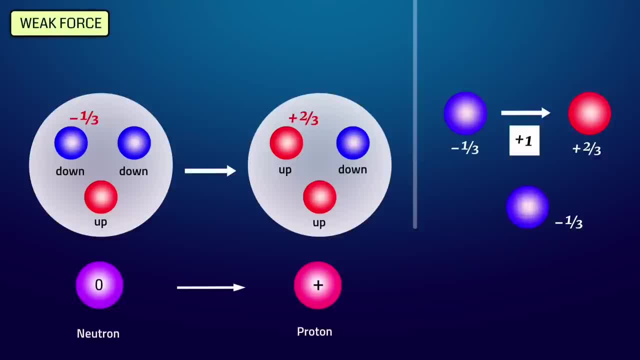 it needs to gain a charge of one down quark or one plus one charge. Now, what does that mean? In order to do that, the down quark emits a w minus boson and becomes a up quark, And what is the function of this? 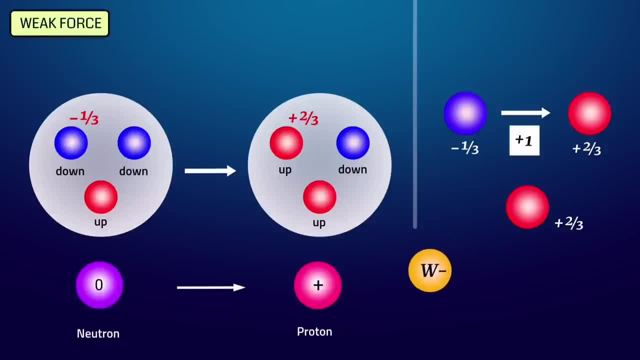 The W minus boson has a Sciences, and so does thepta-boson. it's the�ル, intracore mass times, the H2 and electrostatic force between успite and Larry has a charge of minus 1. So the charge is conserved during this process. but that boson, 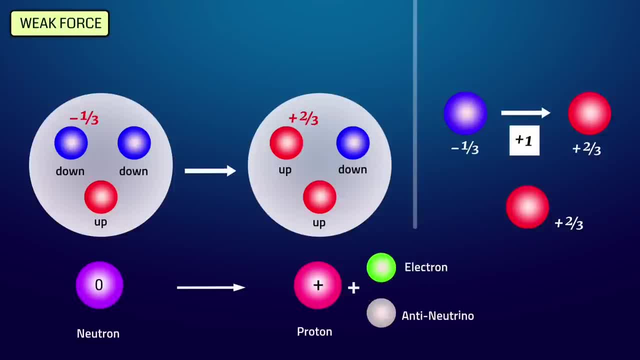 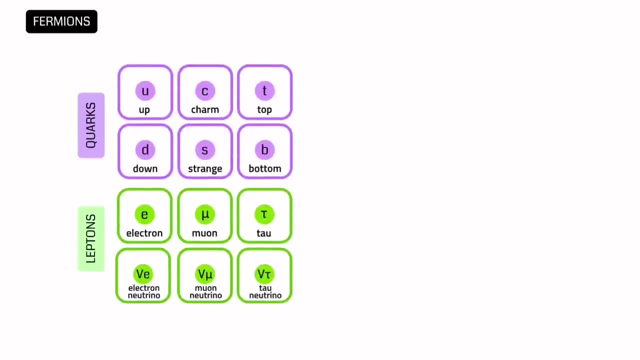 decays very quickly into an electron and an antineutrino pair. An electron has a charge of negative 1 and an antineutrino which has no charge. This is called beta minus decay. But what is an antineutrino? It's an antiparticle. Yes, the fermion group has 12 matter particles and also 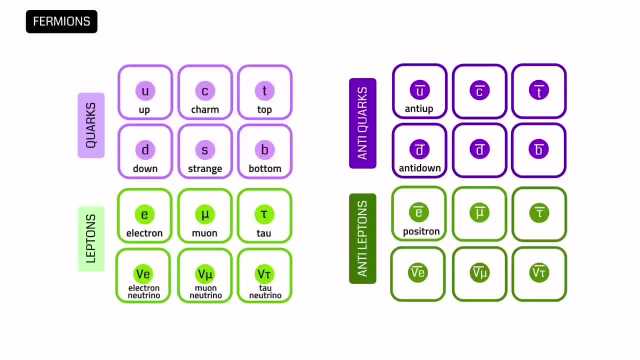 a reactionary 12 antiparticles. The main difference between particles and antiparticles is their opposite charge. For example, electrons have a minus 1 charge, but antielectrons have a plus 1 charge. The other name for an antielectron is positron. However, neutrinos have no charge. 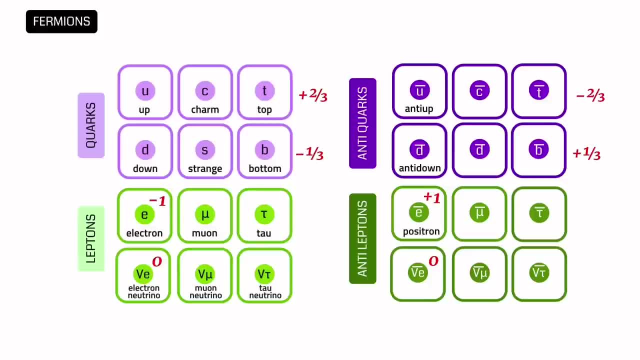 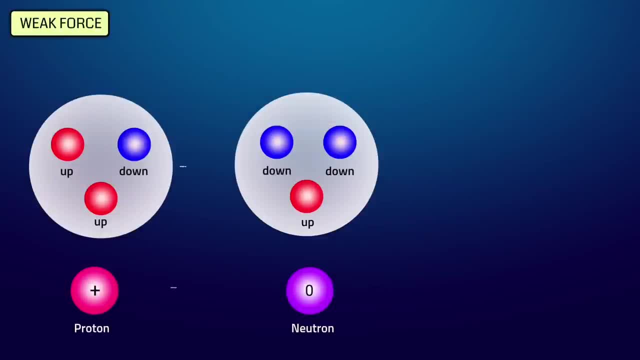 and it remains at zero. So, in order to distinguish between neutrino and antineutrino, the lepton numbers come into play. Similarly, when a proton converts into a neutron, the antineutrino pairs with the neutrinos. So, in order to distinguish between neutrinos and 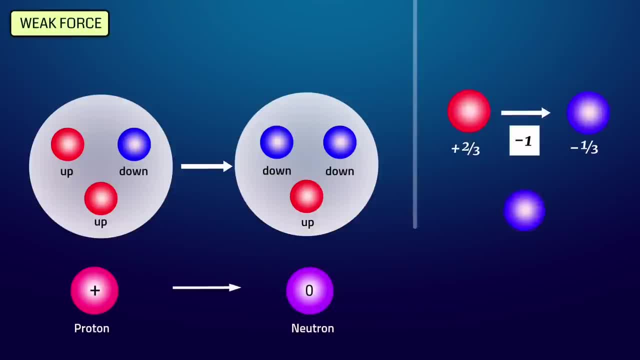 antineutrino, the up quark becomes a down quark. In order to gain the negative charge, it submits a W plus boson. This boson quickly decays into a neutron and a positron, which is called beta plus decay. Without this decay process, hydrogen atoms cannot form helium. 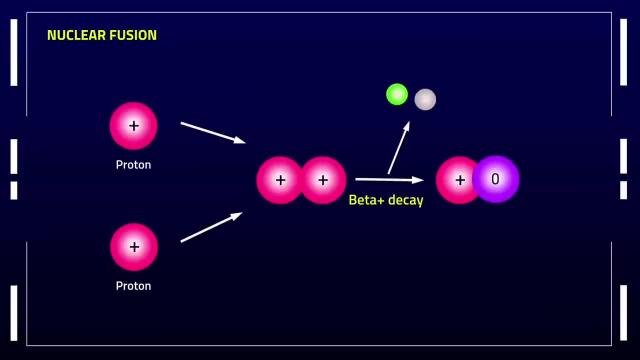 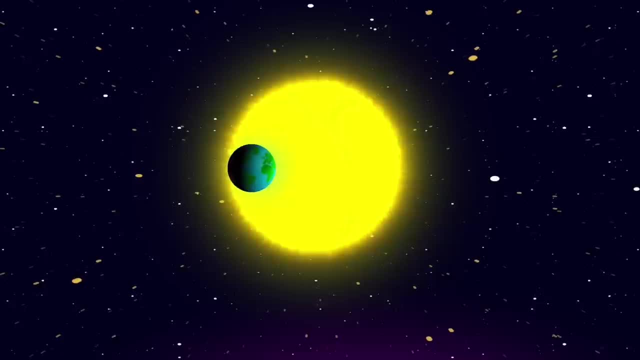 atoms and we can't get energy from this process, which means nuclear fusion would never occur in stars. In our sun, hydrogen atoms turn into helium atoms. This process provides our earth with energy, which is essential for the formation and sustenance of life and 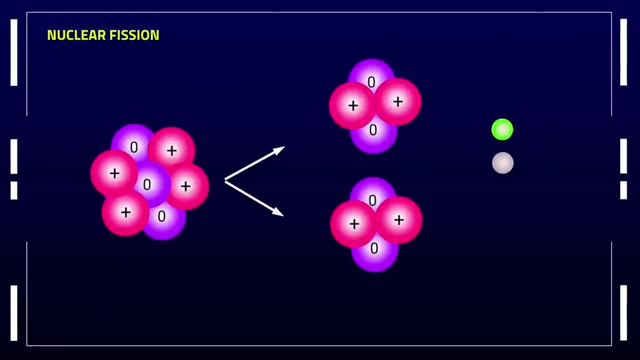 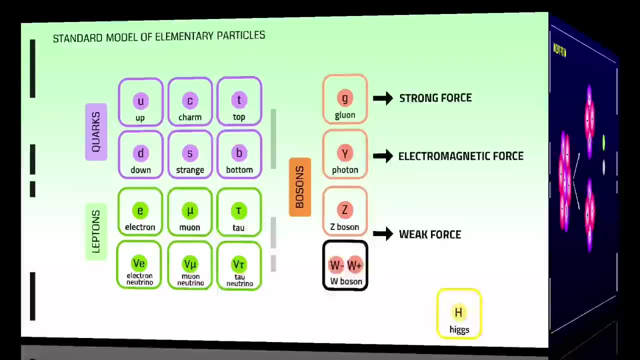 everything else. The same weak force is responsible for nuclear fission. Nuclear fission is when large atoms split into two atoms or release a daughter atom. The other boson involved in the weak interaction is the Z boson. When a particle and an antiparticle 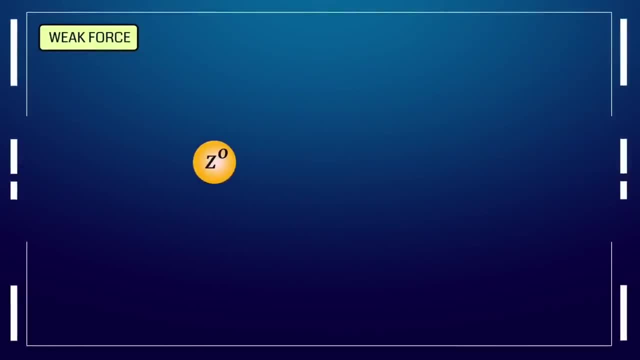 collide, it emits a Z boson and, similar to the W boson, the Z boson decays very quickly, producing another particle, an antiparticle pair. The Z boson's charge is zero, so it only happens between a pair of particles. The Z boson decays very quickly and it emits a Z boson. The Z boson. 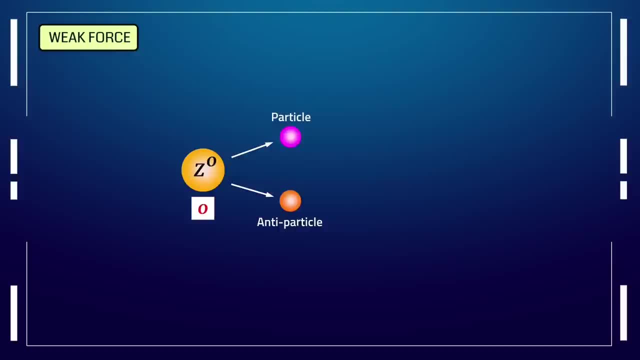 emits a Z boson and, similar to the W boson, the Z boson decays very quickly, producing another particle and antiparticles. The particle and antiparticle pairing together results in a zero charge. For example, an electron has a minus one charge and a positron has a plus one charge, So together 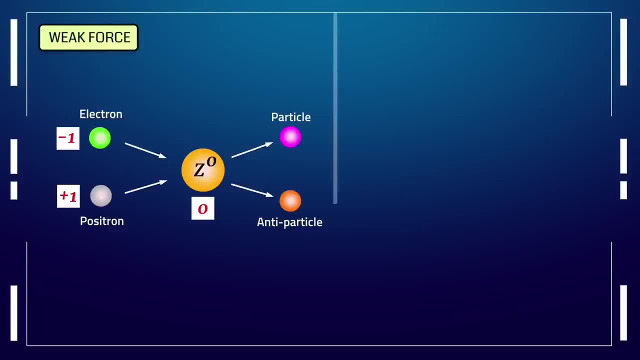 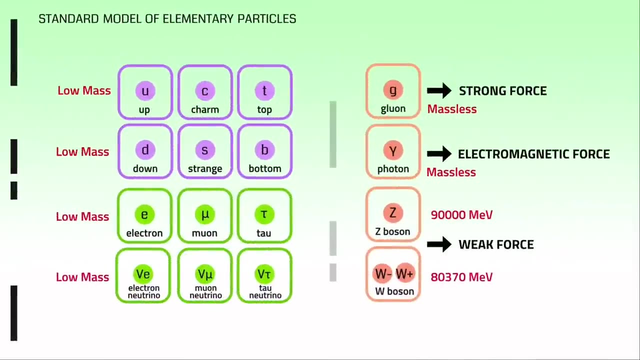 they become zero charged, the Z boson. And if we look at the meson, it contains one quark and an antiquark. so it decays into a Z boson and quickly becomes other particles. The reason why W and Z bosons decay quickly is because of their mass, which is very high compared to fermions. But why? 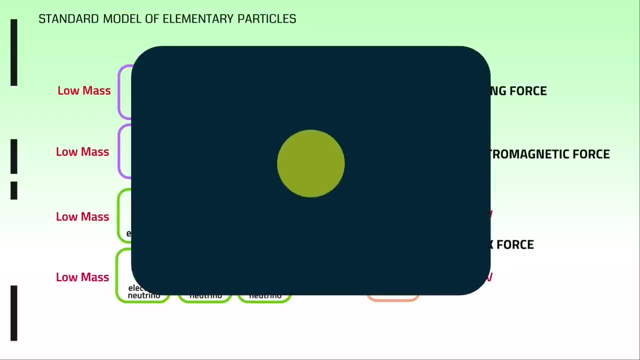 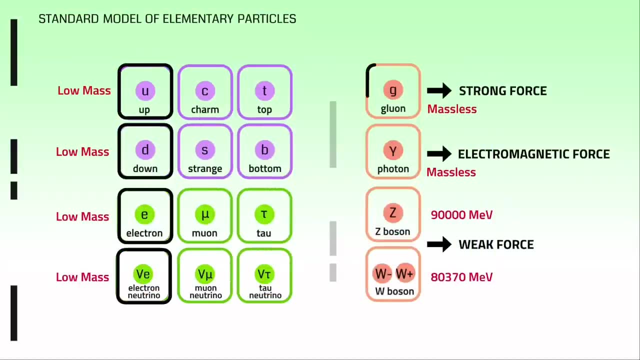 is it called a weak force? Because its range is very, very small, Smaller than a proton. If we look deeper, in the standard model, our first generation particles, gluons and photons, have a long time life. A proton has a lifespan of 10 to the power of 34 years. 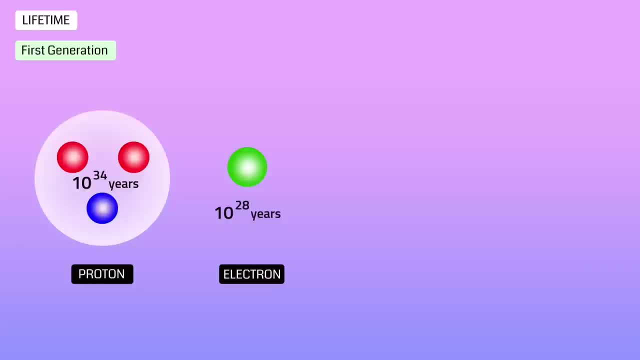 and an electron 6.6 into 10 to the power of 28 years. On the other hand, W and Z bosons have a lifetime of 10 to the power of 24 years And an electron 6.6 into 10 to the power of 28 years. 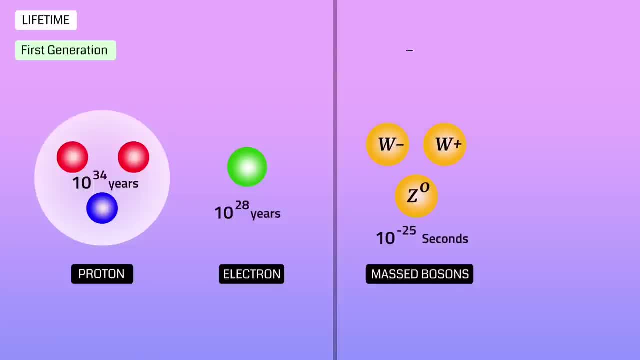 of just 10 to the power of minus 25 seconds, and the second generation particle, the muon, lasts 10 to the power of minus 6 seconds. So, due to their very short lifetimes, these are only detectable in particle accelerators. 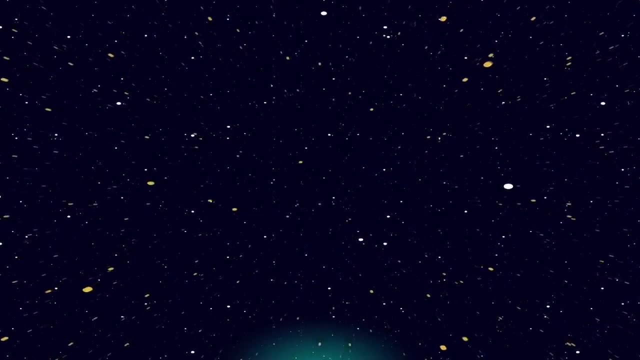 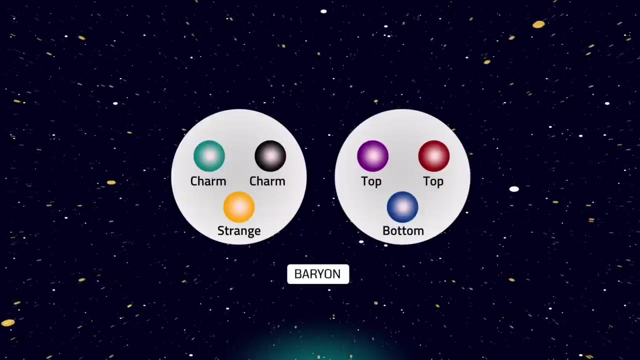 Only the first generation particles are involved in forming most of the matter in the universe. However, we can create baryon particles made up of the second or third quarks, But these all have much greater mass and decay very rapidly into protons and neutrons. However, we don't 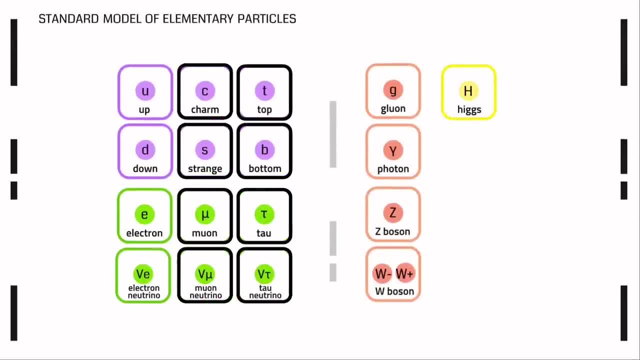 yet know exactly why the remaining two generation particles exist and quickly end their lifetimes, And the other one that has a place in the standard model is the Higgs boson, or the Higgs field, which is believed to be responsible for the mass of an elementary particle, and the Z and W bosons.